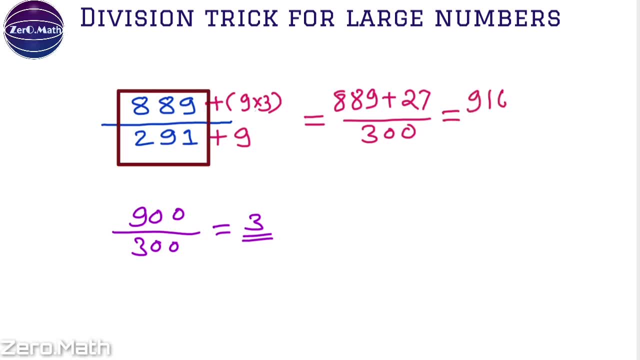 is equal to 916 by 300.. If you solve this equation, you will get answer as 3.0533 and so on. So the resulting answer is 1.039448.. ДиммеJe superior and heart is equivalent to 11 musical. 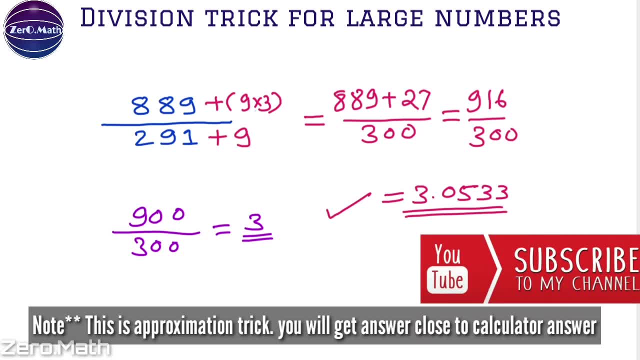 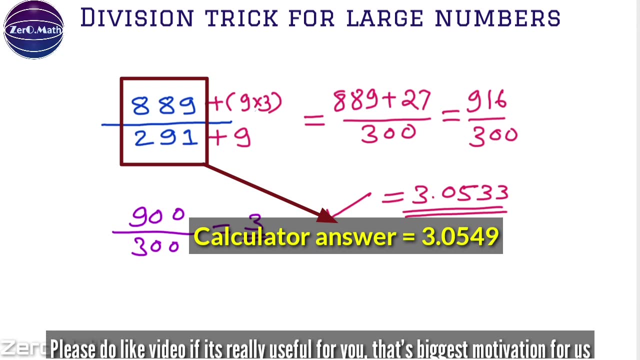 travaillеs in a section of a case for on and off the linguistic Kalimba. So adding 9 times. this is the answer. However, please note this answer is approximate answer. If you try to find out the answer of this sum with the calculator, you will get answer as 3.0549.. You can see both. 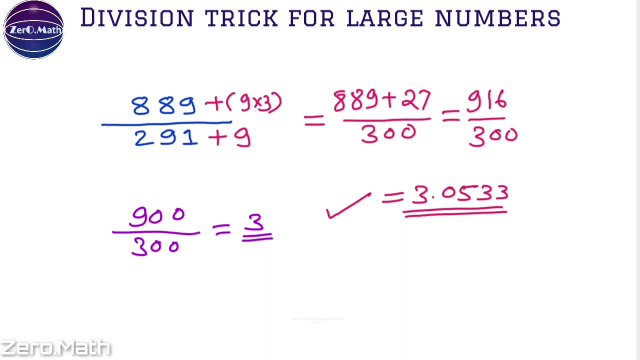 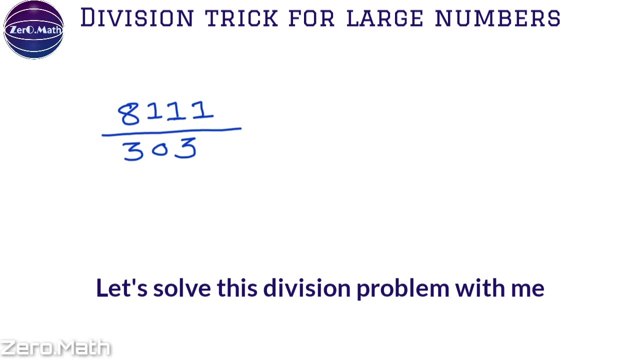 the answers are almost similar. This trick is useful in the exam, where you have to solve such sum very quickly. Let us take another example. Let us solve 8111 by 303.. Try to solve this example along with me. Again, we will try to simplify our denominator. So to simplify this. 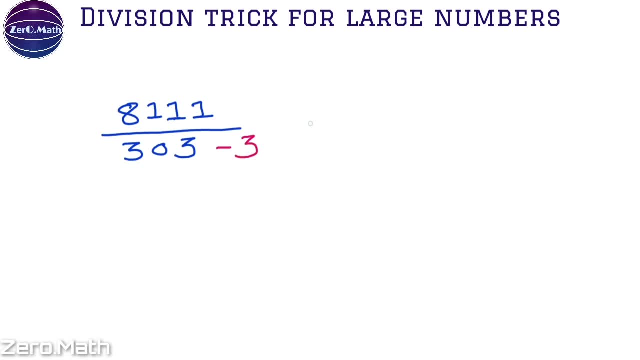 I will subtract 3 from 303 so that it will become 300.. If I am subtracting 3 from my denominator, what should I subtract from my numerator Exactly? This is the question. So let us try to find out the approximate unit value of this equation. 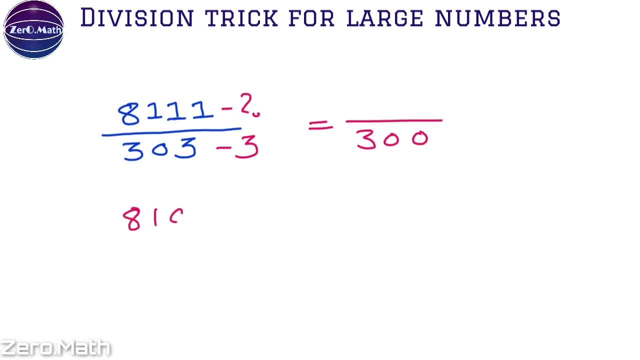 So 8111, I can write approximate value as 8100 and 303 can be approximated as 300. So if we divide this we will get 27 as the approximate unit value. So which means my numerator is 27 times my denominator. So if I am subtracting 3 from my denominator, 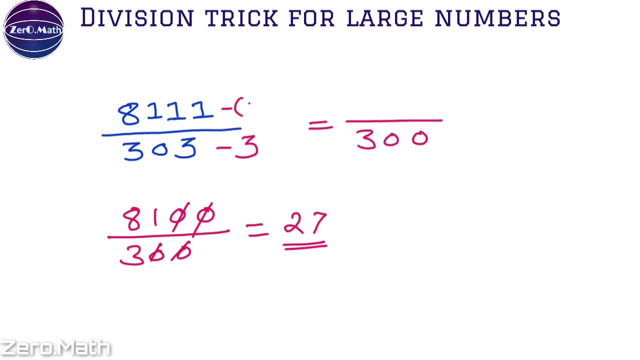 I should be subtracting 3 times 27 from my numerator, So value of my numerator will be 8111 minus 27 times 3 is 81, which is equal to 8030 by 300.. If you solve this equation, 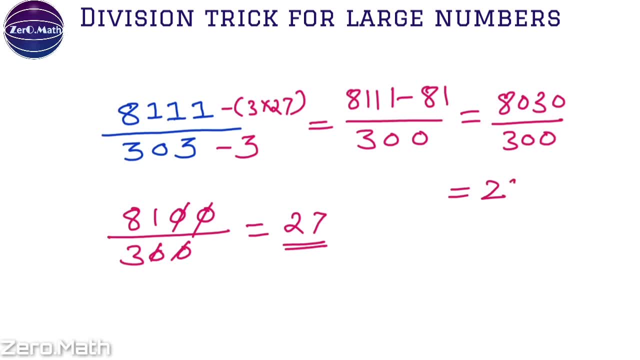 you will get answer as 26.30.. So the answer is 26.766, which is my answer. If you try to find out the answer of this equation with the calculator, the answer will be 26.768.. So you can see, both the answers are almost same. 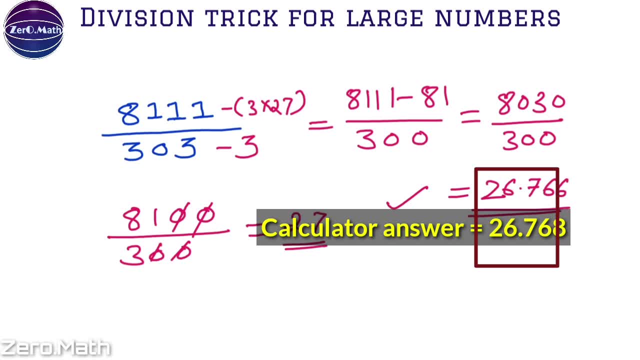 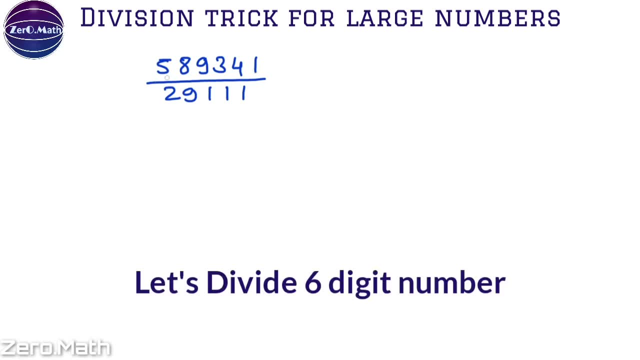 If you approximate, you will get absolutely the same answer, that is, 26.76.. Let us take a complicated example now and let us try to divide this six-digit number. In such example, where the number of digits are more, we will convert the numerator to the. 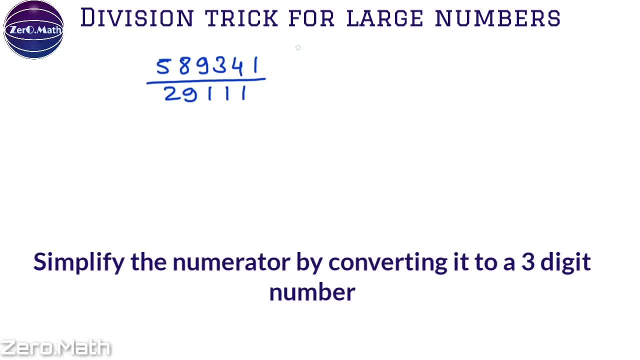 three-digit number for simplification purpose by removing the remaining digits. So let us remove three digits from the numerator so that it will become 589.. Since we are removing three digits from the numerator, let us remove the three digits from the denominator as well. So my denominator. 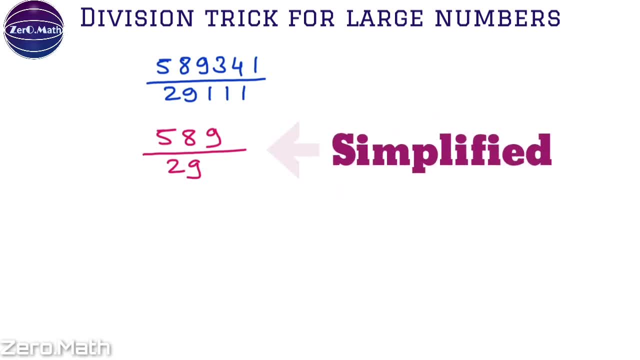 will become 589 by 589.. So what it will look like is this: 4Ч1, which called as 4τ9 slash 4Ç1, and then the denominator will be 4τ3 towards 5τ2.. So my denominator will include: 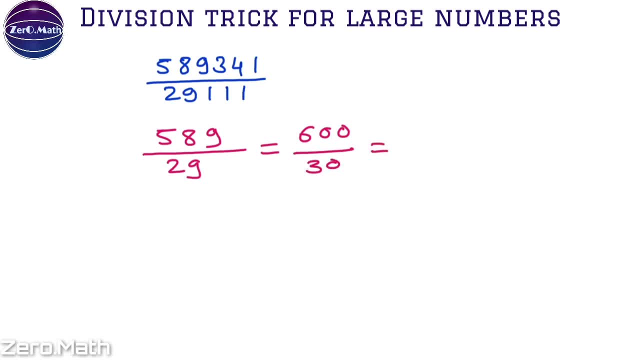 these開心 units, and then I will take a daily verge and I will make the also. So let us do this: 5τ9ะ and 5τ3 becomes about 6, such that this is 4τ2 plus 4τ3 plus 5τ2.. 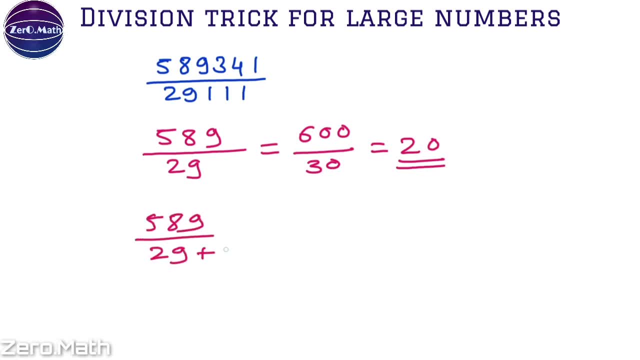 Now what will be the answer here? Let us find out. Let us say 0.. Let us say 0.. Let us see denominator. since I am adding 1 to the denominator, I will add 1 times 20 to the numerator, so it will. 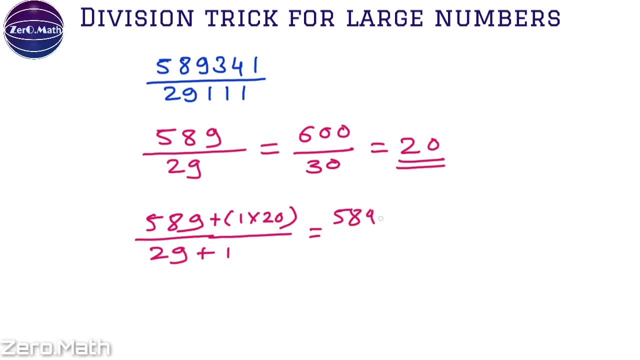 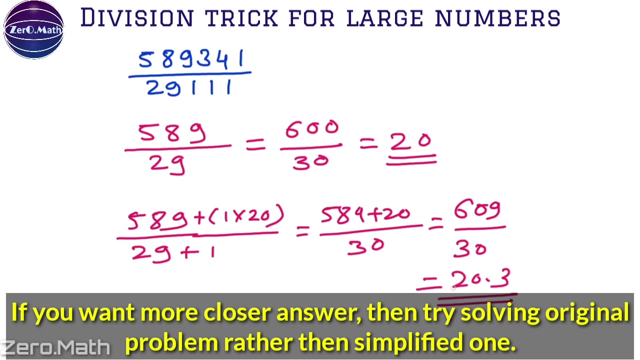 become 589 plus 20 by 30, which is equal to 609 by 30, which will give the answer as 20.3. this is the approximate answer. if you want more closer answer and if you have enough time in examination for the same, then we would recommend to solve the original problem rather than solving the simplified. 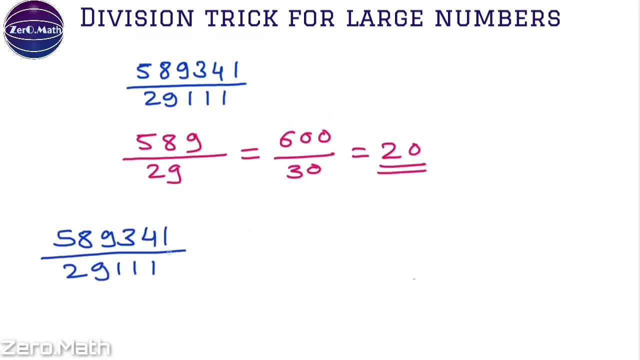 one solve the original problem statement. now, if I add 889 to the denominator, my denominator will become 30,000, so it's easy to divide by 30,000. since I am adding 1 to the denominator, I will add 1 to the denominator, so it's easy to divide by 30,000. 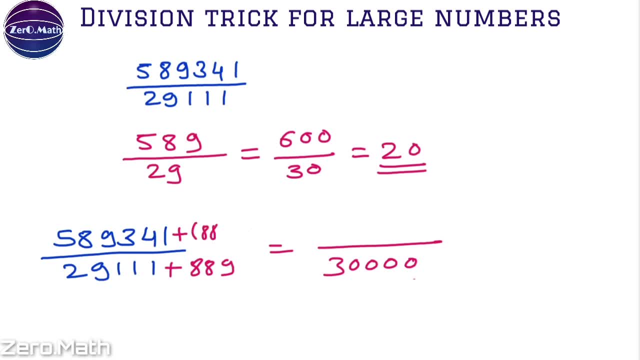 since I am adding 1 to the denominator, I will add 1 to the denominator. I will add 1 to the denominator. adding 889 to the denominator, I should be adding 889 times 20, which is my unit value, to my numerator, so it will become 589341. plus 889 times 20 will be 1700 and 780. so let's add this, we'll get 607121 by. 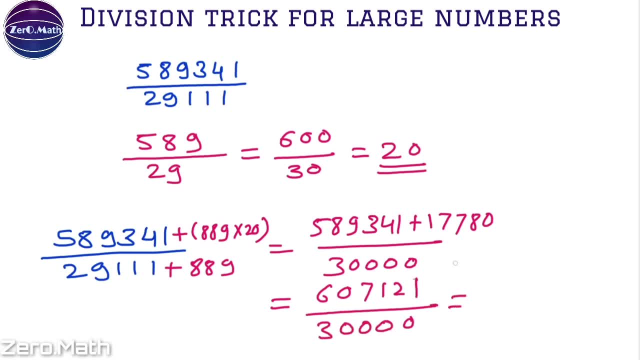 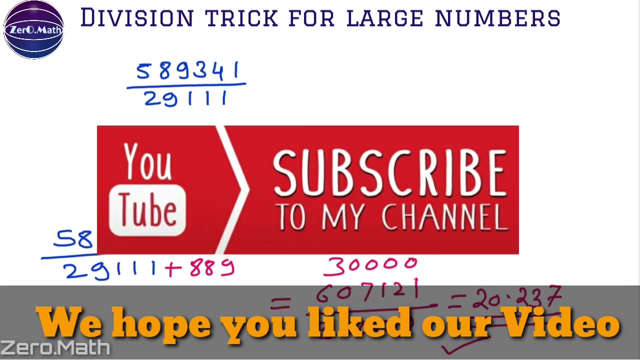 30000, which will give you answer as 20.237, which will be much closer to the calculator answer. so calculator answer is 20.24 in this case. friends, I hope you like this video. if you like this video, please do not forget to subscribe our channel and keep in touch with us for more videos like this. 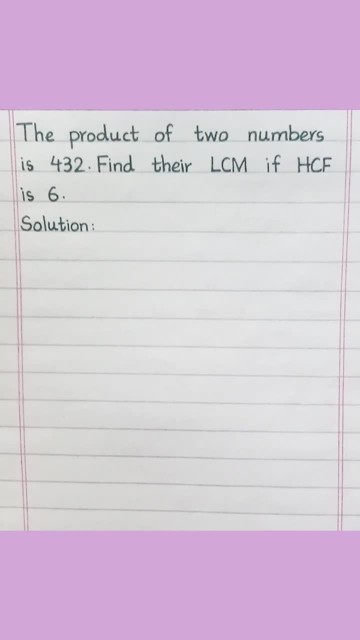 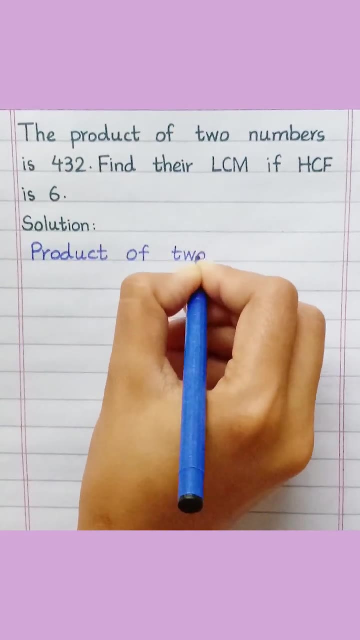 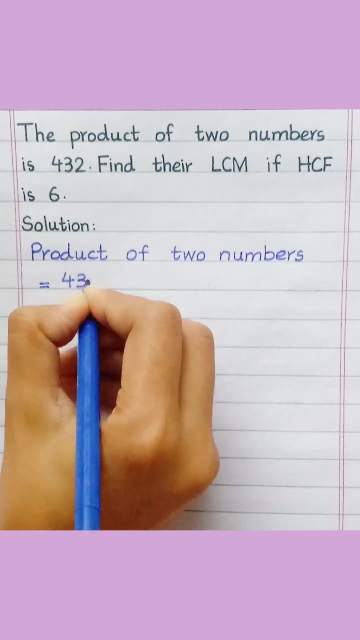 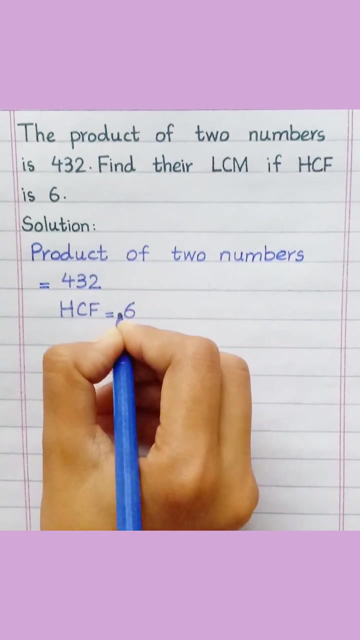 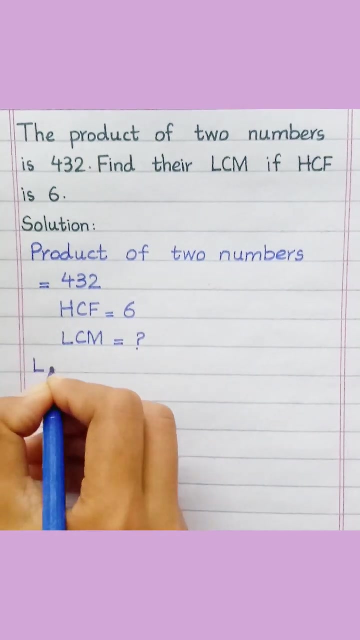 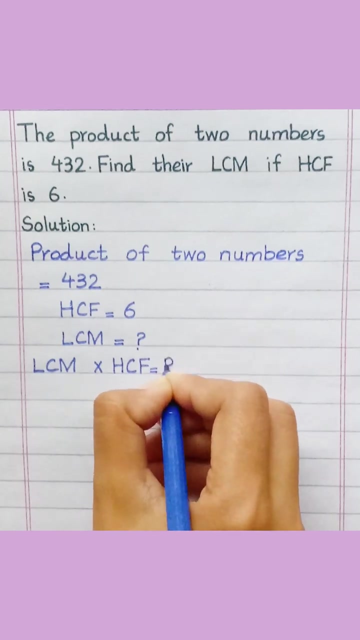 The product of two numbers is 432.. Find their LCM if HCF is 6.. Solution: Product of two numbers equal 432.. HCF equal 6.. Find LCM: LCM multiply HCF: equal product of two numbers. 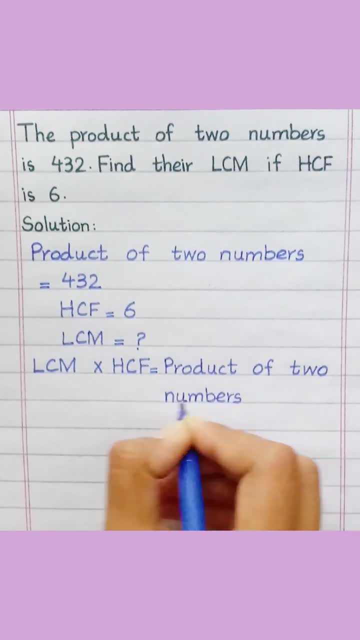 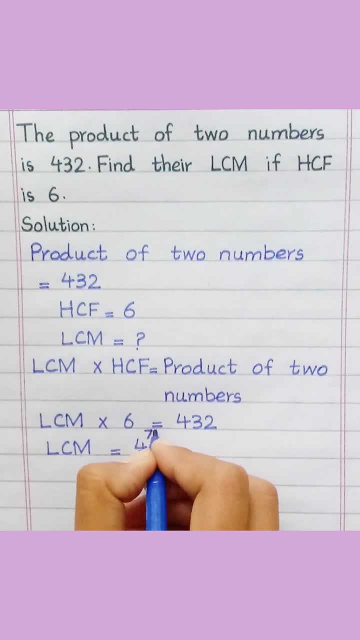 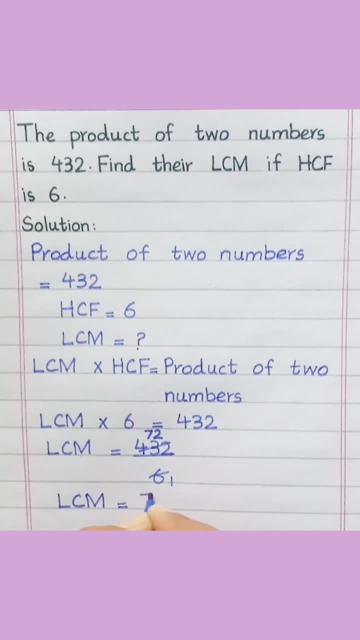 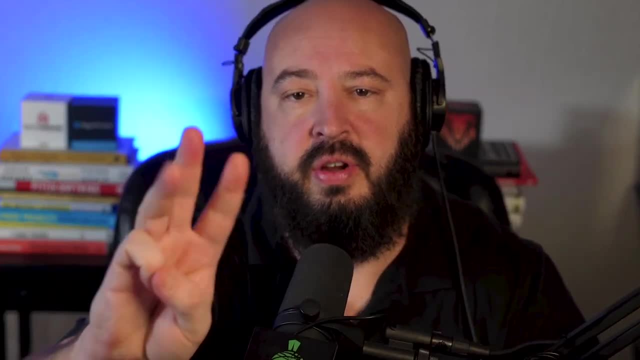 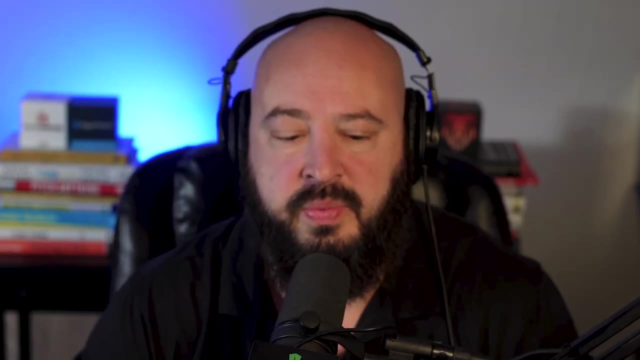 This is the BiggerPockets Podcast Show 936.. What's going on, everyone? This is David Green, your host of the BiggerPockets Real Estate Podcast, Joined today, as always with Rob Abasolo Delighted to be here, my friend, bringing real estate knowledge to the people.